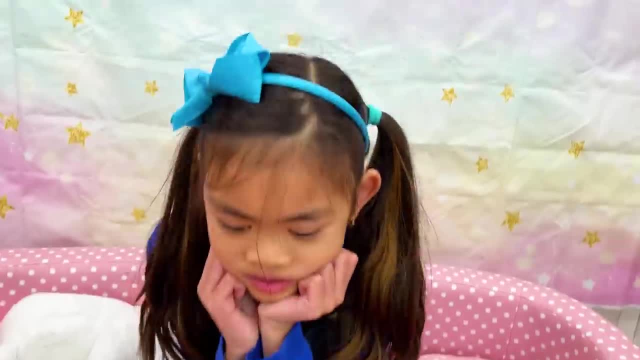 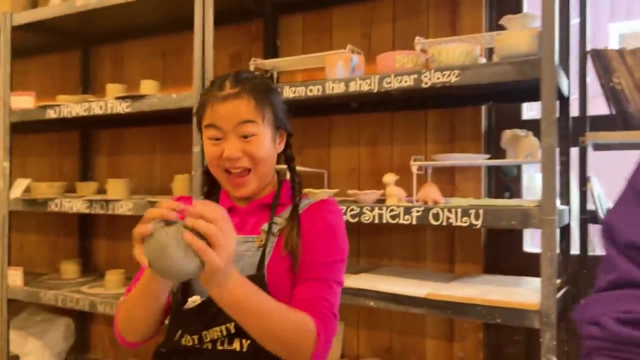 All my favorite vases are broken. Aw, Aw, We're so sorry. Ah, I have an idea. Huh, We're gonna make clay and pottery. Yay, Yay, Yay, Yay, Yay, Yay. 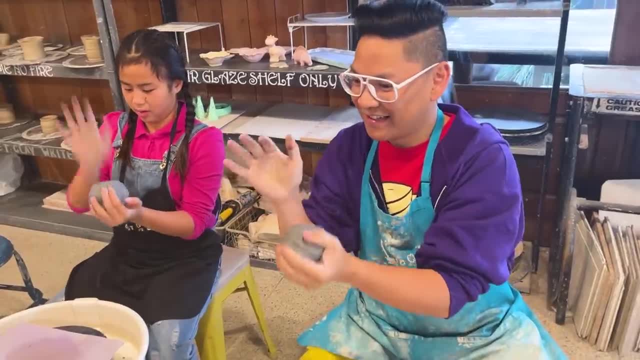 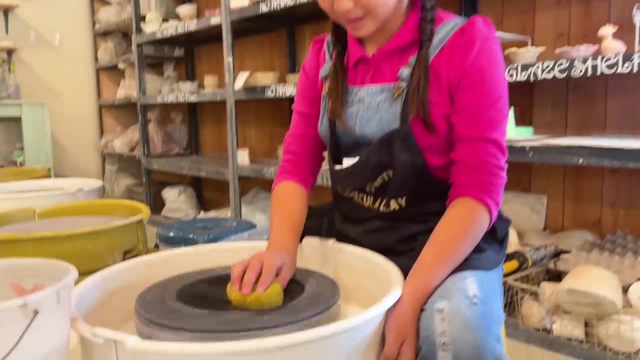 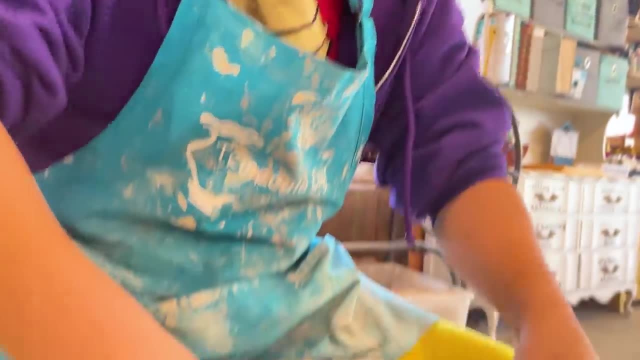 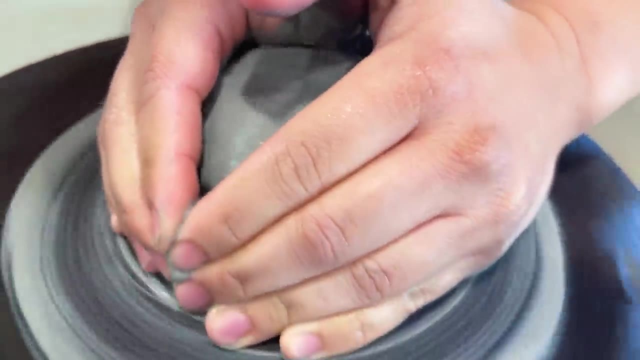 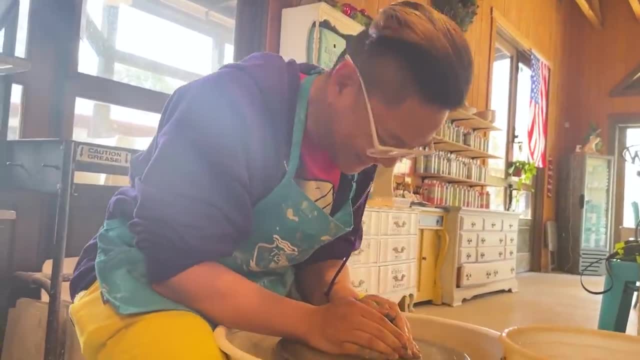 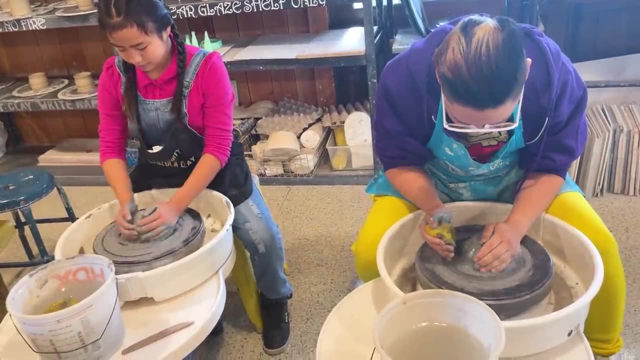 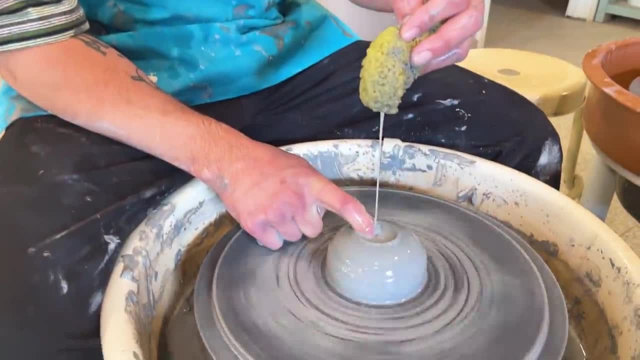 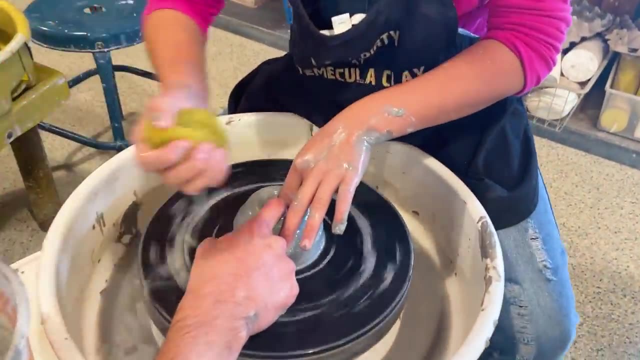 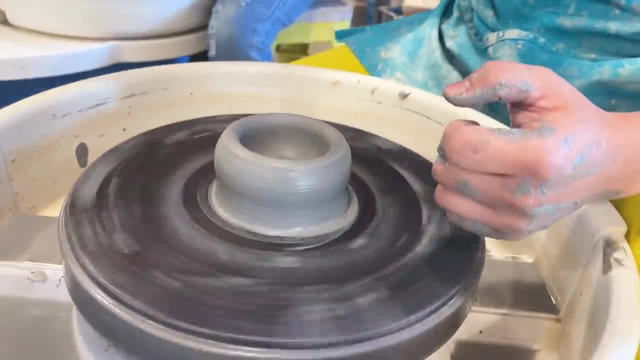 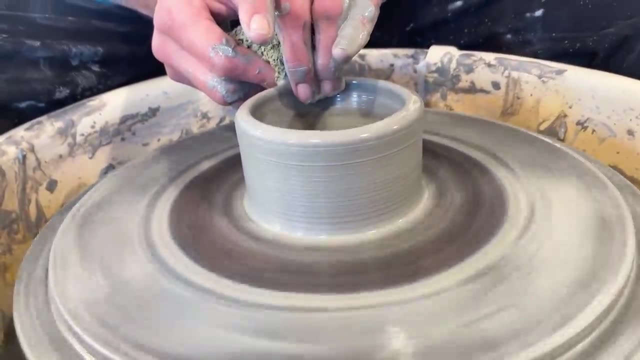 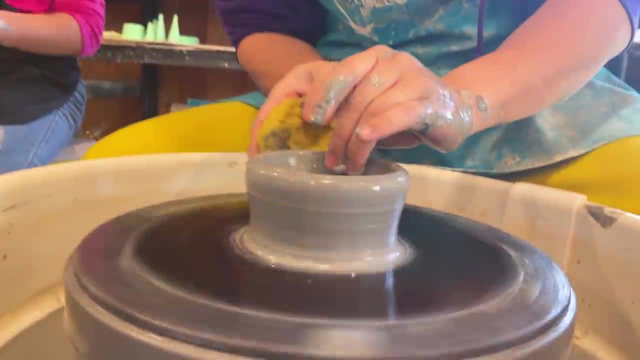 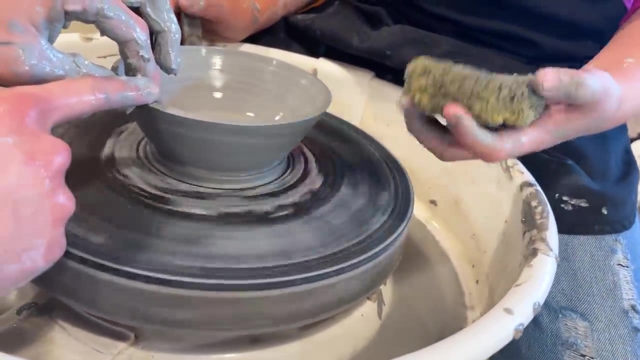 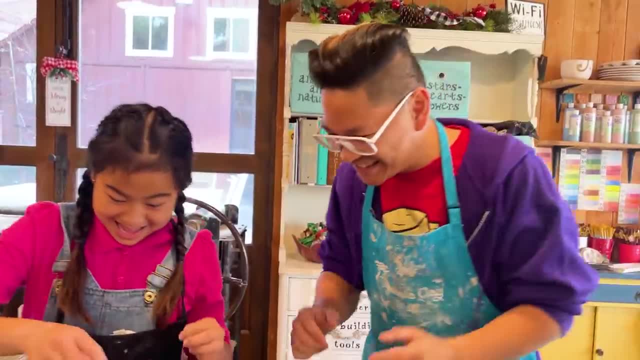 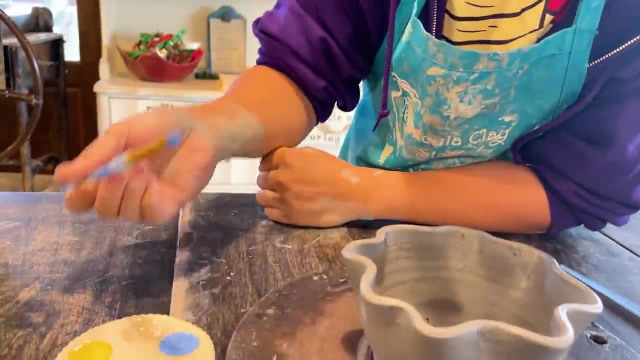